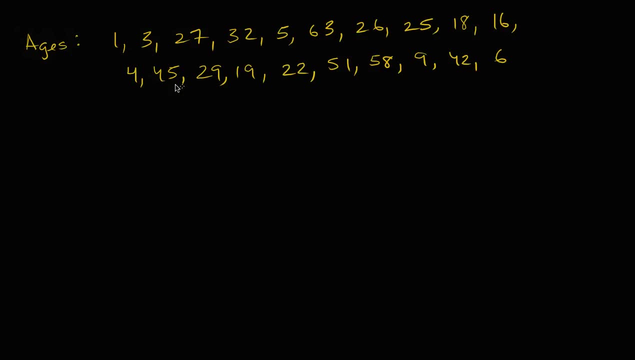 And so when you just look at these numbers, it really doesn't give you a good sense of it. It's just a bunch of numbers, And so how could you do that? Well, one way to think about it is is to put these ages into different buckets. 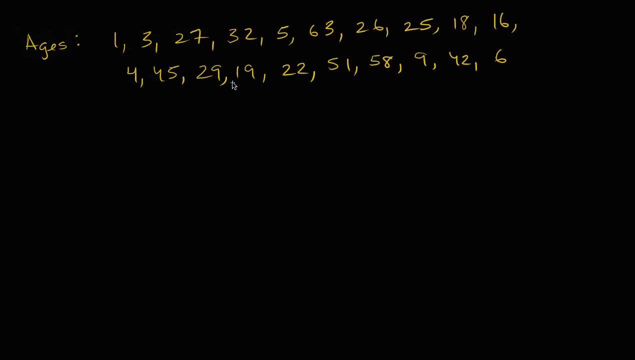 and then to think about how many people are there in each of those buckets, Or sometimes someone might say how many in each of those bins. So let's do that, So let's do buckets or categories, So I like sometimes it's called a bin. 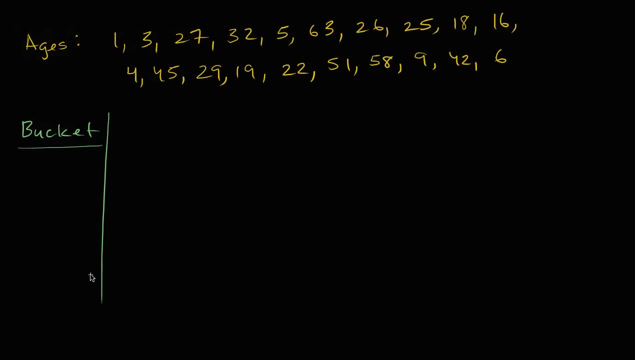 So the bucket- I like to think of it more of as a bucket: The bucket and then the number in the bucket, The number in the bucket Number. I'll just write the number whoops. It's the whoops. 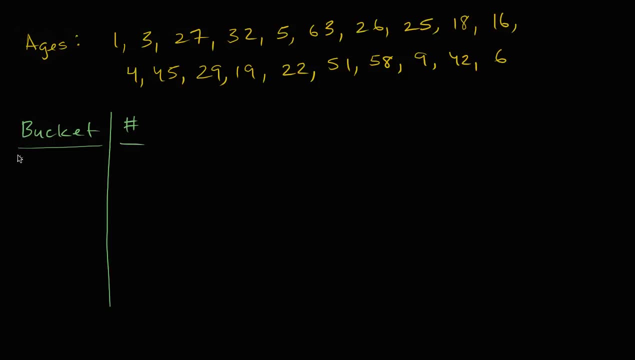 It's the number, It's the number in the bucket. All right, so let's just make buckets. let's make them 10-year ranges, So let's say the first one is ages zero to nine. So how many people? and then we just define all of the buckets here. 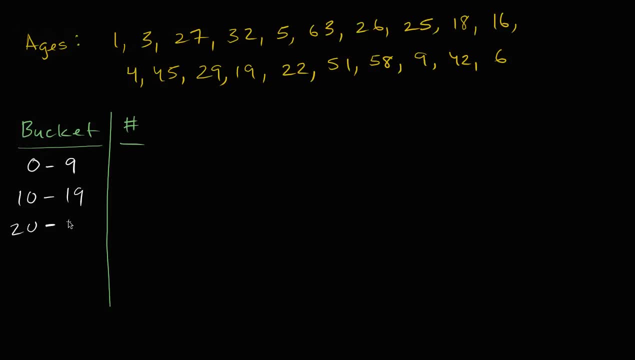 So the next one is ages 10 to 19,, then 20 to 29,, and 40 to 49,, 50 to 59. Let me make sure you can read that properly. And then you have 60 to 69.. 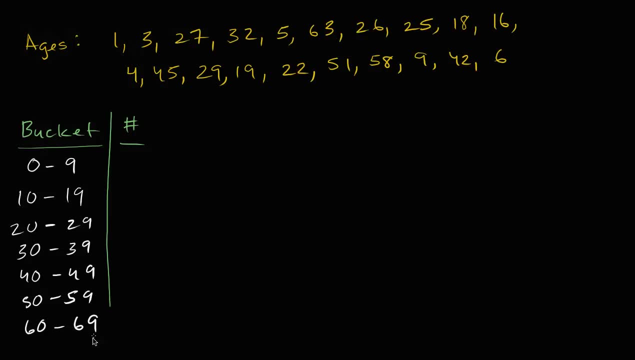 And I think that covers everyone. I don't see anyone 70 years old or older here. So then, how many people fall into the zero to nine-year-old bucket? Well, it's gonna be one, two, three, four, five, six people fall into that bucket. 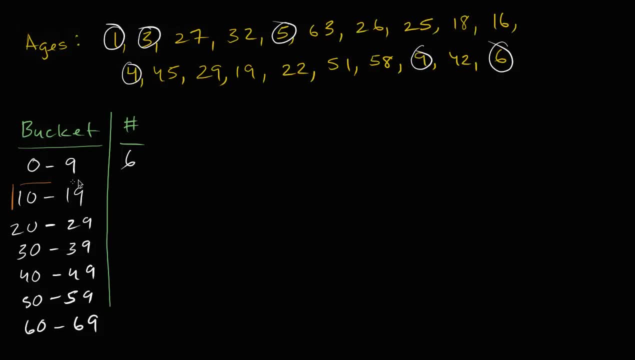 How many people fall into the? how many people fall into the 10 to 19-year-old bucket? Well, let's see One, two, three, Three people, And I think you see where this is going. What about 20 to 29?? 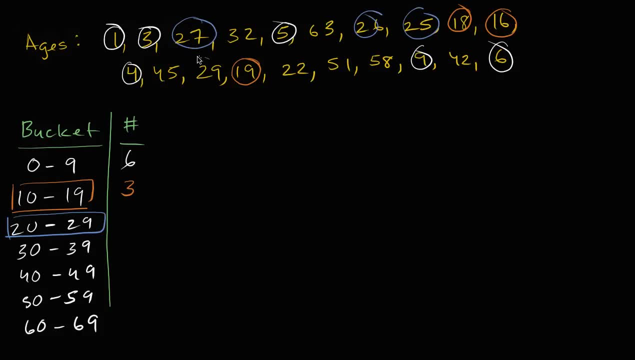 So it's one, two, three, four, five people. Five people fall into that bucket, All right. what about 30 to 39?? We have one and that's it. only one person in that 30 to 39? 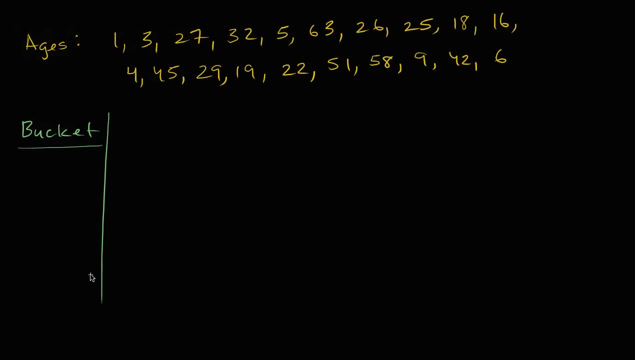 So the bucket- I like to think of it more of as a bucket: The bucket and then the number in the bucket, The number in the bucket Number. I'll just write the number whoops. It's the whoops. 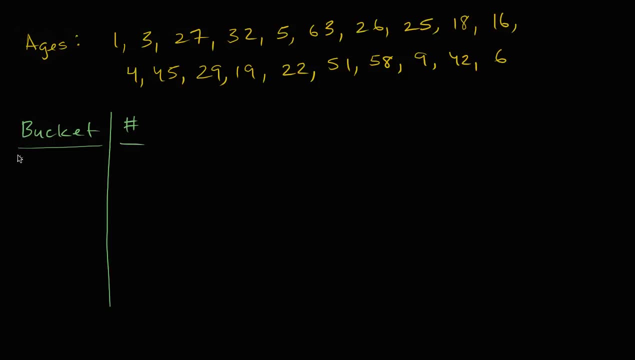 It's the number, It's the number in the bucket. All right, so let's just make buckets. let's make them 10-year ranges, So let's say the first one is ages zero to nine. So how many people? and then we just define all of the buckets here. 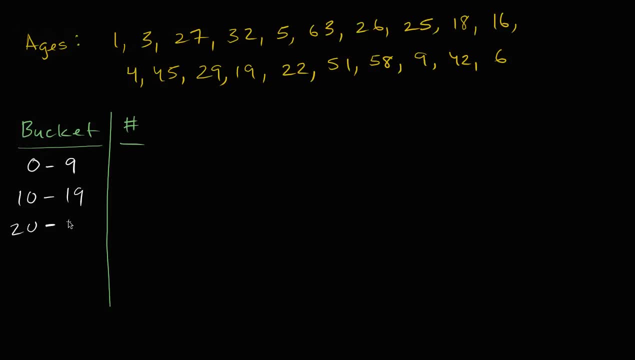 So the next one is ages 10 to 19,, then 20 to 29,, and 40 to 49,, 50 to 59. Let me make sure you can read that properly. And then you have 60 to 69.. 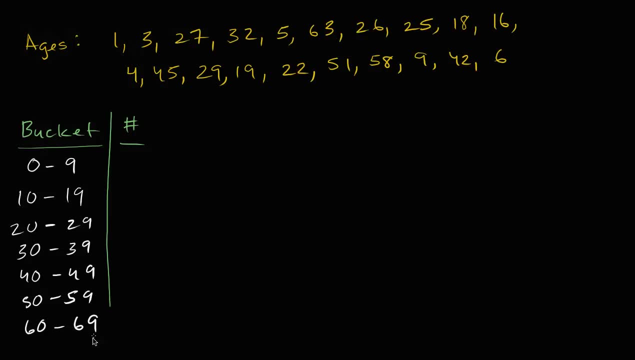 And I think that covers everyone. I don't see anyone 70 years old or older here. So then, how many people fall into the zero to nine-year-old bucket? Well, it's gonna be one, two, three, four, five, six people fall into that bucket. 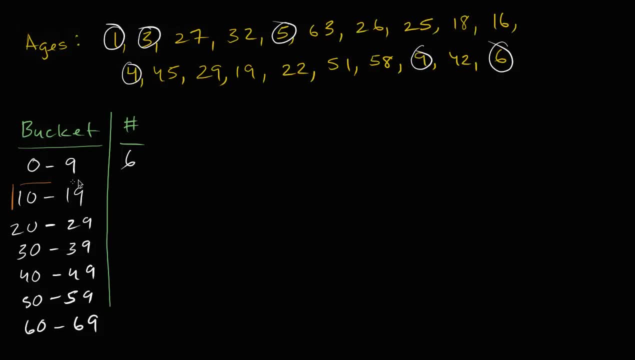 How many people fall into the? how many people fall into the 10 to 19-year-old bucket? Well, let's see One, two, three, Three people, And I think you see where this is going. What about 20 to 29?? 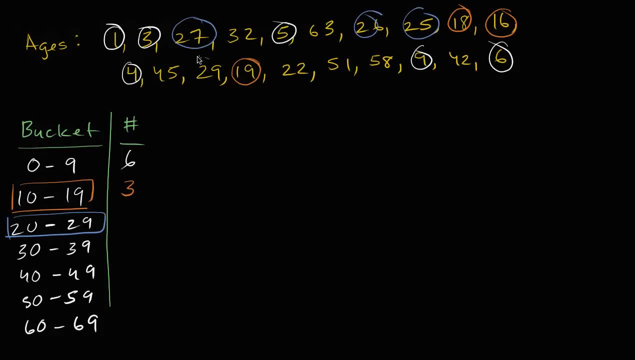 So it's one, two, three, four, five people. Five people fall into that bucket, All right. what about 30 to 39?? We have one and that's it, only one person in that 30 to 39 bin or bucket or category. 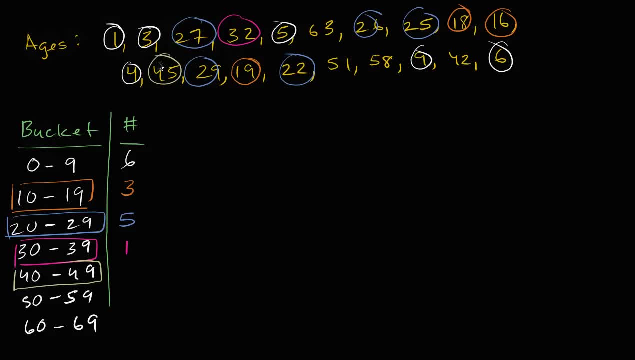 All right, what about 40 to 49?? We have one, two people, Two people are in that bucket- And then 50 to 59. So you have one, two people, Two people And then finally, finally, ages 60 to 69,. 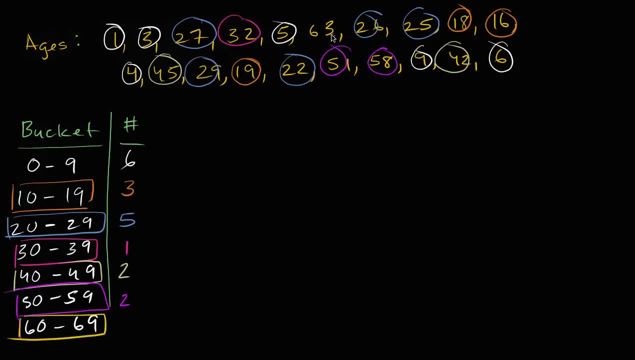 let me do it in a different color. 60 to 69,. There is one person right over there. So this is one way of thinking about how the ages are distributed, but let's actually make a visualization of this And the visualization that we're gonna create. 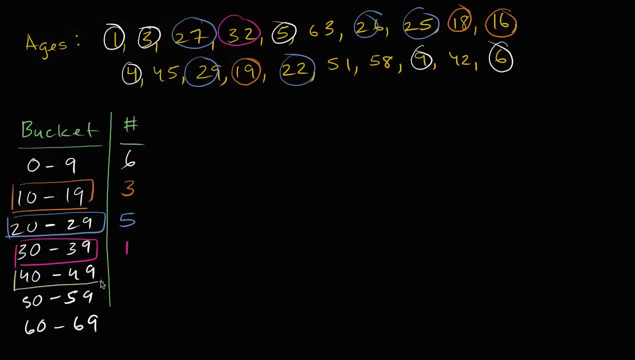 bin or bucket or category. All right, what about 40 to 49?? We have one, two people, Two people are in that bucket, And then 50 to 59. So you have one, two people, Two people And then finally, finally, ages 60 to 69.. 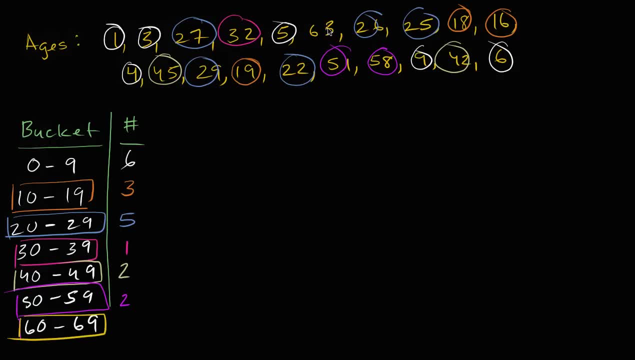 Let me do it in a different color: 60 to 69. There is one person right over there, So this is one way of thinking about how the ages are distributed, but let's actually make a visualization of this And the visualization that we're gonna create. 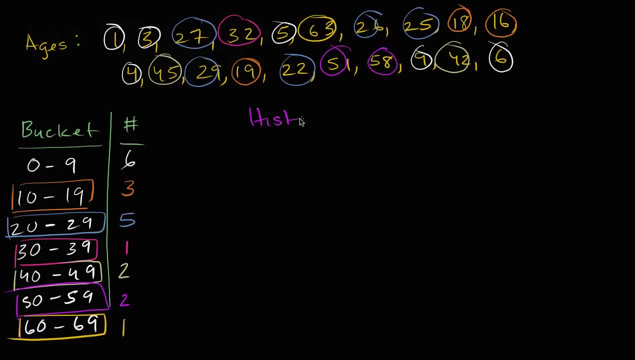 this is called a histogram, Histogram, Histogram. We're taking data that can take on a whole bunch of different values. We're putting them into categories. then we're gonna plot how many folks are in each category. How big are each of those? 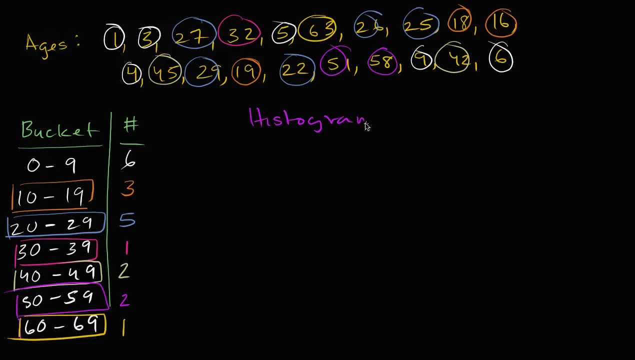 How big are each of those categories? And actually I wrote histogram, I wrote histogram, I should have written histogram, So a histogram, So let's do this All right. So on this axis, let's see: the largest category has six. 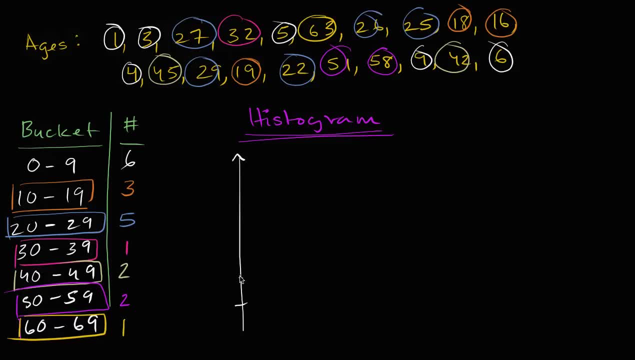 So this is the number, Number of folks- And it's gonna go: one, two, three, four, five, six. One, two, three, four, five, six. This is the number And on this axis it's gonna be the buckets. 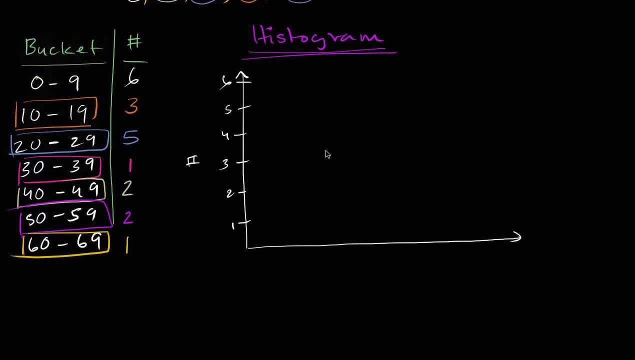 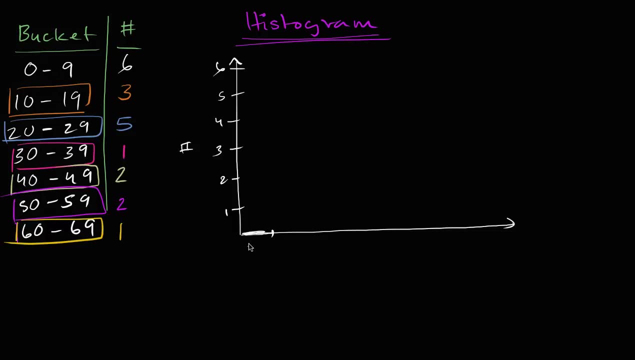 The buckets And let me scroll up a little bit. Now that I have my data here, I don't have to look at my data set again. So I have one bucket. This is going to be the zero to nine bucket Right over here. 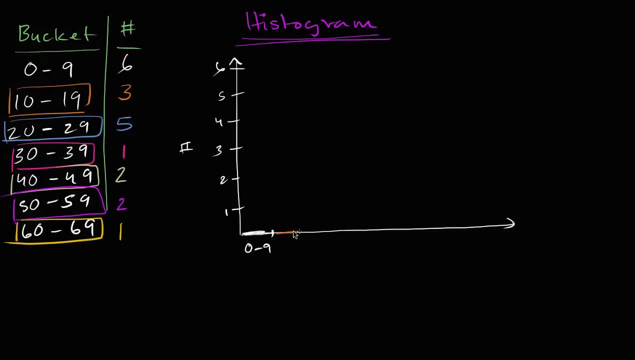 Zero to nine, Then I'm going to have the three. Actually, let me just plot them, Since I have my pen that color. So in zero to nine, there are six people. Zero to nine, there are six people. So I'll just plot it like that. 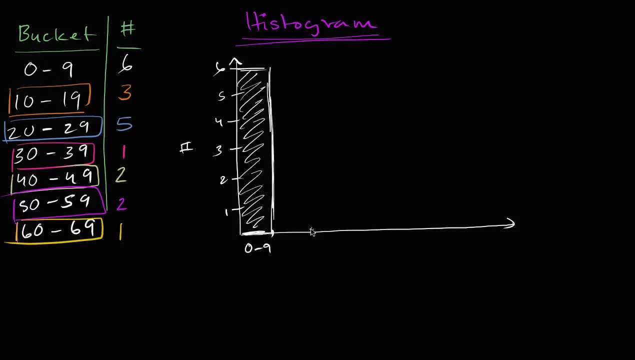 And then we have the 10 to 19.. There are three people, So 10 to 19,. there are three people, So I'll do a bar like this. Then 20 to 29,. I have five people, 20 to 29, which is gonna be this one. 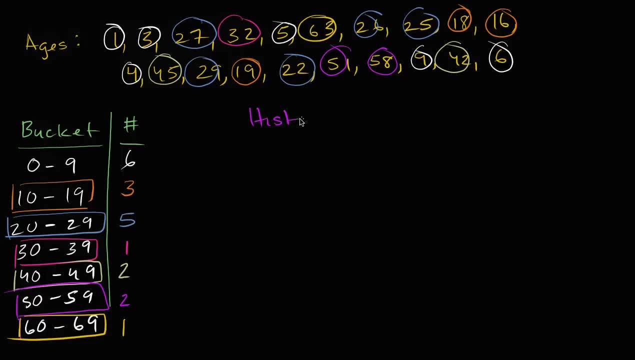 this is called a histogram. Histogram, We're taking data that can take on a whole bunch of different values. we're putting them into categories. then we're gonna plot how many folks are in each category. how big are each of those? how big are each of those categories? 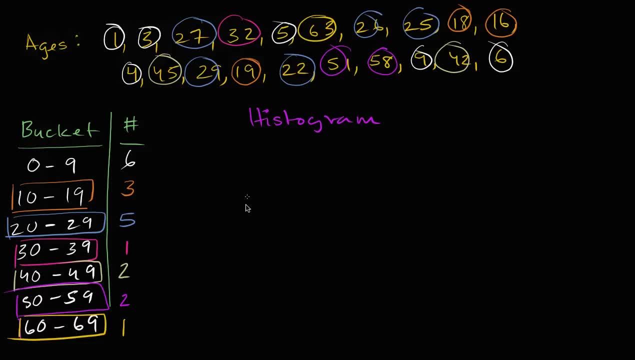 And actually I wrote histogram. I wrote histogram. I should have written histogram, So a histogram, So let's do this All right. So on this axis, let's see: the largest category has six. So this is the number. 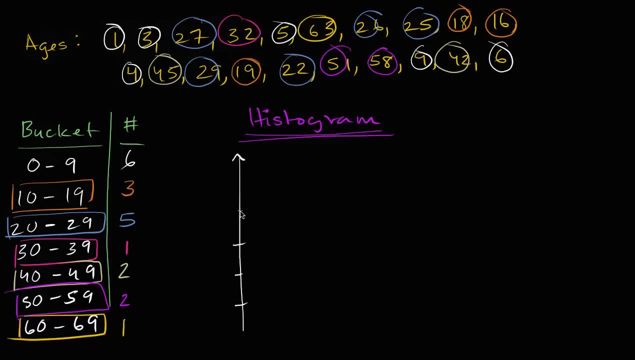 Number of folks and it's gonna go: one, two, three, four, five, six. One, two, three, four, five, six. This is the number And on this axis I'm gonna make the buckets, The buckets. 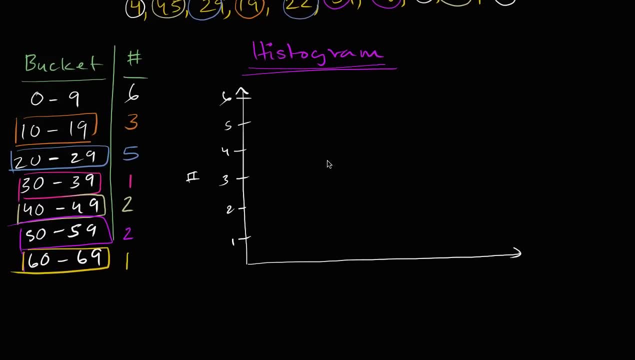 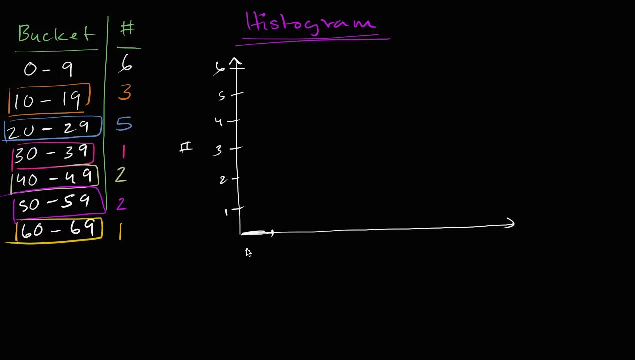 And let me scroll up a little bit. now that I have my data here, I don't have to look at my data set again. So I have one bucket. This is going to be the zero to nine bucket Right over here: Zero to nine. 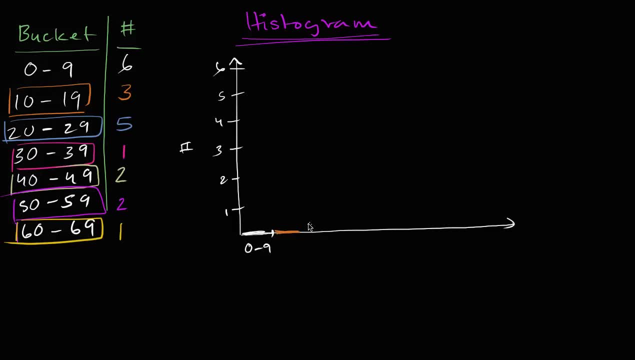 Then I'm going to have the three. actually let me just plot them, since I have my pen that color. So zero to nine, there are six people. Zero to nine, there are six people. So I'll just plot it like that. 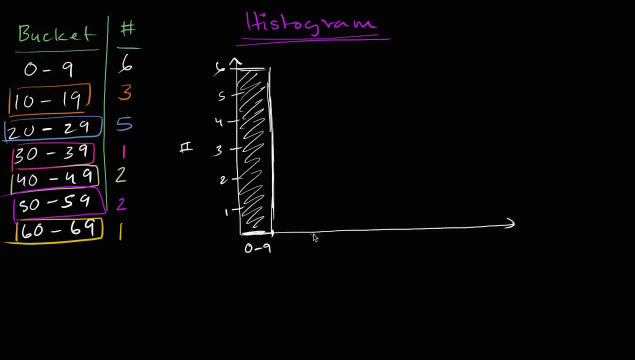 And then we have the 10 to 19.. There are three people, So 10 to 19,. there are three people, So I'll do a bar like this. Then 20 to 29,. I have five people, 20 to 29, which is gonna be this one. 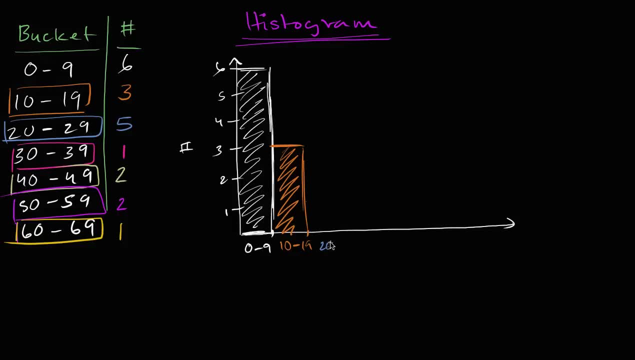 which is getting. I'm writing too big. So 20 to 29,. this is gonna be this bar. There's five people, Five people there, So it'll look like this. I should have made the bars wide enough so I could write below them. 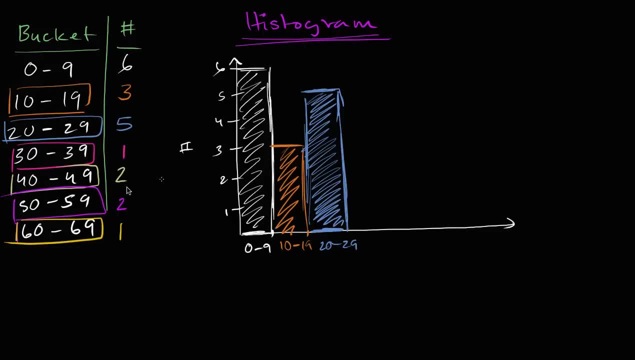 but I've already that train has already left. All right. All right, then, 30 to 39, I'll try to write smaller: 30 to 39, that's gonna be this bar. right over here We have one person. 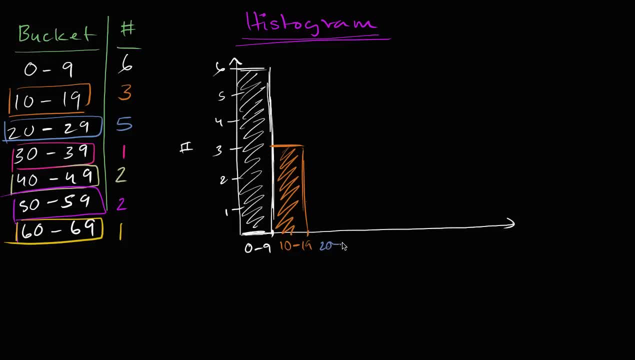 which is getting. I'm writing too big. So 20 to 29,. this is gonna be this bar. There's five people, Five people there, So it'll look like this. I should have made the bars wide enough so I could write below them. 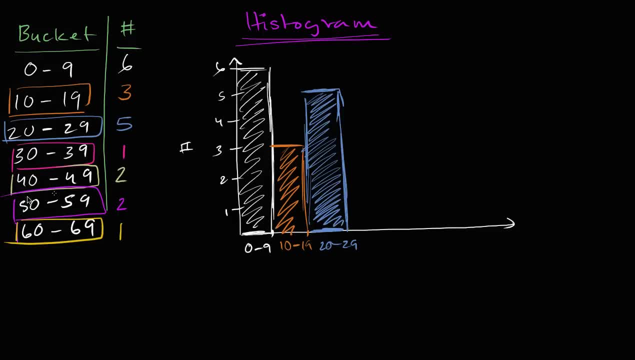 but I've already that train has already left. All right. All right, then, 30 to 39.. I'll try to write smaller: 30 to 39.. That's gonna be this bar. right over here We have one person. 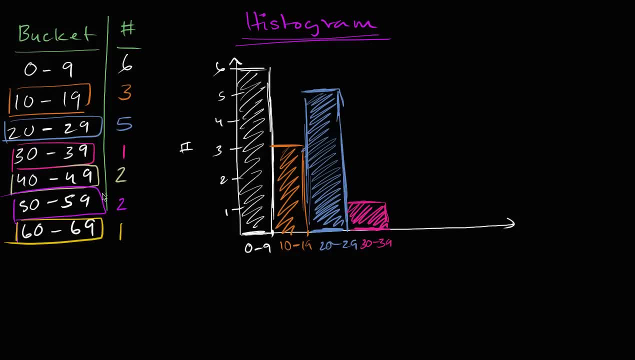 One person, And then we have 40 to 49.. We have two people: 40 to 49,, two people. So it looks like this: 40 to 49,, two people, Almost there, 50 to 59, we have two people. 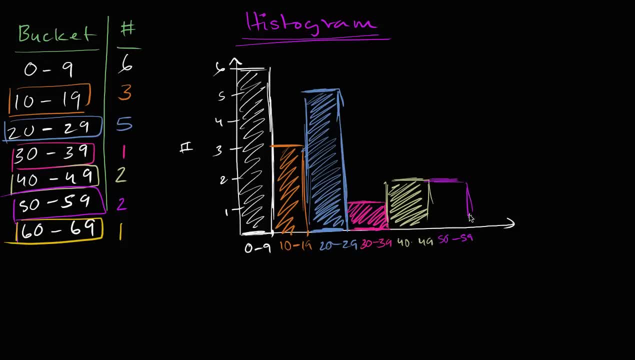 50 to 59,: we also have two people. So that's that right over there. That's this category. And then finally, 60 to 69,: we have one person. 60 to 69,: we have one person. 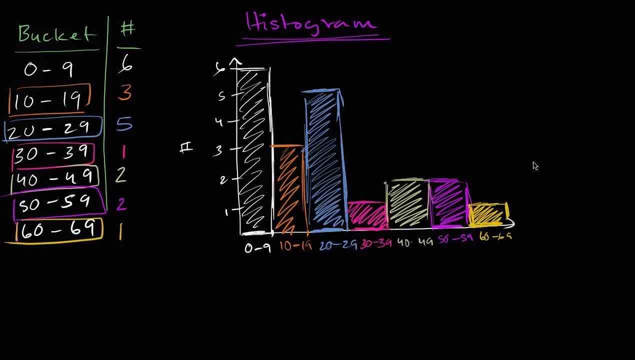 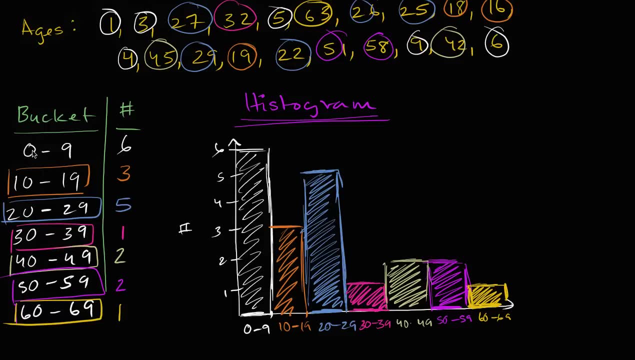 We have one person And what I have just constructed. I took our data. I took our data, I put it into buckets that are kind of representative of the categories I care about. Zero to nine is kind of young kids, 10 to 19, I guess you could call them adolescents. 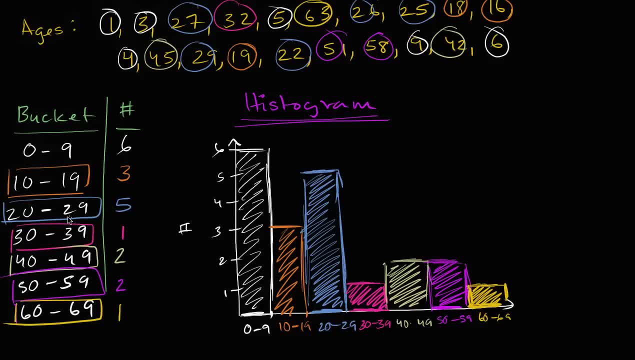 or roughly teenagers- although obviously if you're 10, you're not quite a teenager yet- And then all the different age groups, And then when I counted the number in each bucket and I plotted it, now I can visually get a sense of how the age is distributed in this restaurant. 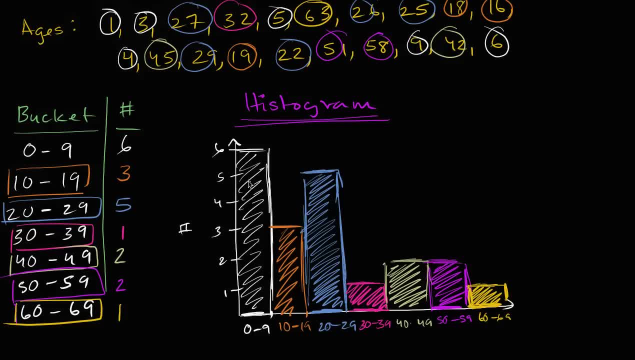 This must be some type of a restaurant that gives away toys or something, because there's a lot of younger people. Maybe it's very family friendly, so every adult that comes in, maybe there's a lot of young adults with kids and or maybe grandparents up here. 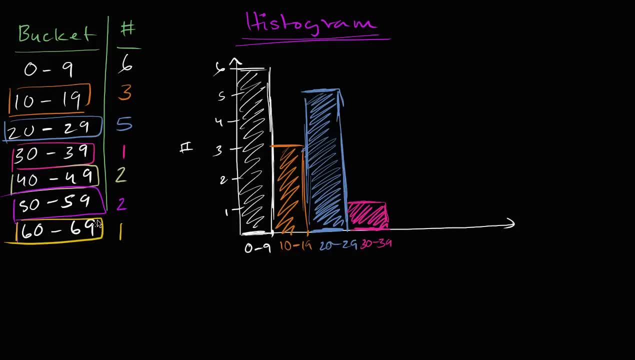 One person, And then we have 40 to 49.. We have two people: 40 to 49,, two people. So it looks like this: 40 to 49,, two people, Almost there, 50 to 59, we have two people. 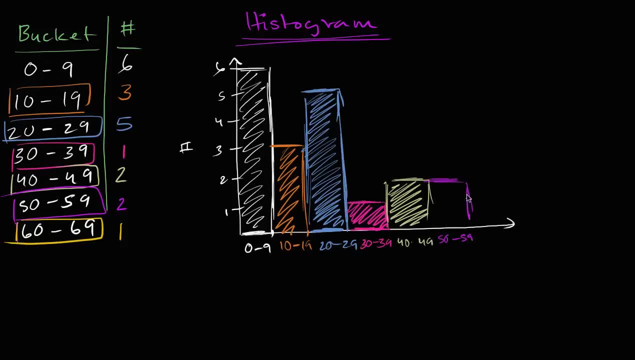 50 to 59,: we also have two people. So that's that right over there. That's this category. And then finally, 60 to 69,: we have one person. 60 to 69,: we have one person. 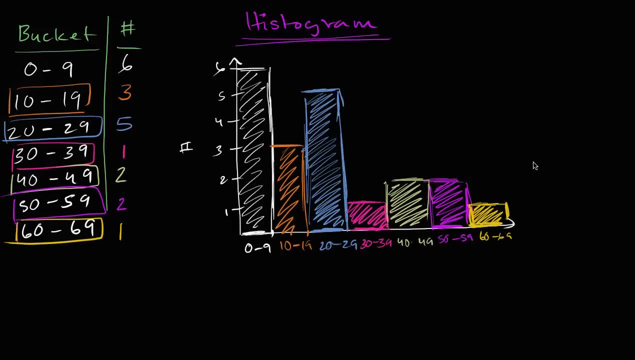 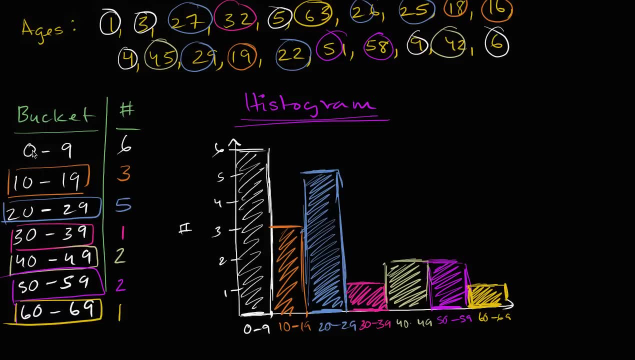 We have one person And what I have just constructed. I took our data. I took our data, I put it into buckets that are kind of representative of the categories I care about. Zero to nine is kind of young kids, 10 to 19, I guess you could call them adolescents. 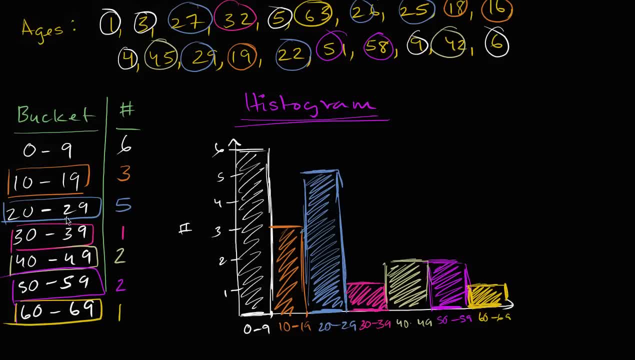 or roughly teenagers- although obviously if you're 10, you're not quite a teenager yet- And then all the different age groups, And then when I counted the number in each bucket and I plotted it, now I can visually get a sense of how the age is distributed in this restaurant. 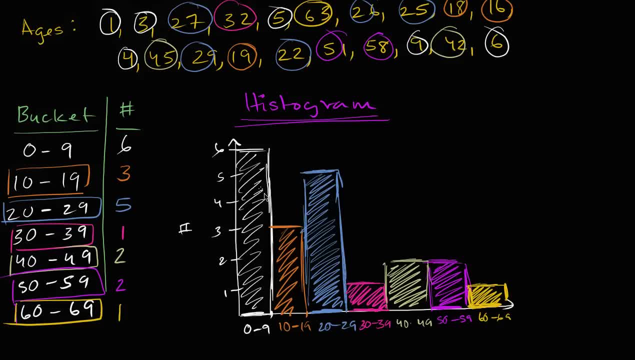 This must be some type of a restaurant that gives away toys or something, Because there's a lot of younger people. Maybe it's very family friendly, So every adult that comes in, maybe there's a lot of young adults with kids or maybe grandparents up here. 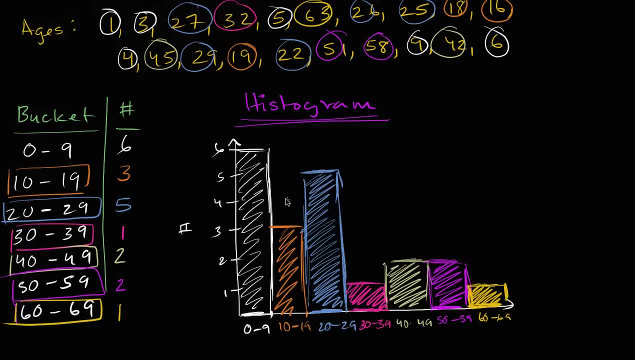 and they just bring a lot of kids to this restaurant. So it gives you a view of what's going on here. Just a lot of kids here, a lot fewer senior citizens. So once again, this is just a way of visualizing things. 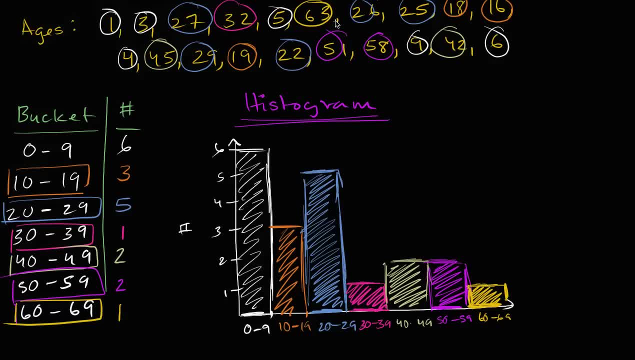 We took a lot of data. that can take multiple data points, Instead of plotting each data point like we might do in a dot plot. instead of saying how many one-year-olds are there, Well, there's only one one-year-old- How many three-year-olds are there? 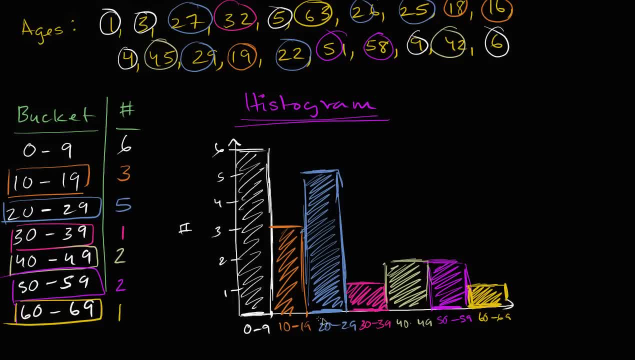 There's only one three-year-old. That wouldn't give us much information. We would just have these single dots if we were doing a dot plot, But as a histogram we're able to put them into buckets And we're just like hey. generally between ages zero and nine. 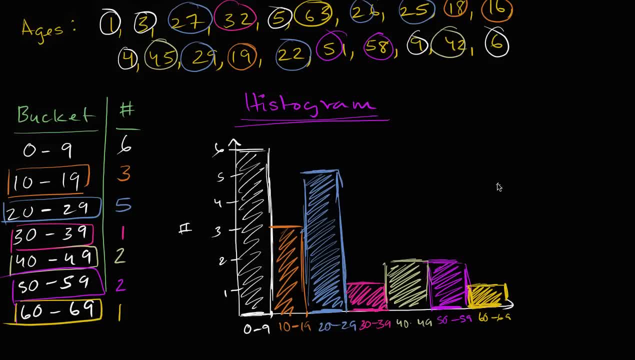 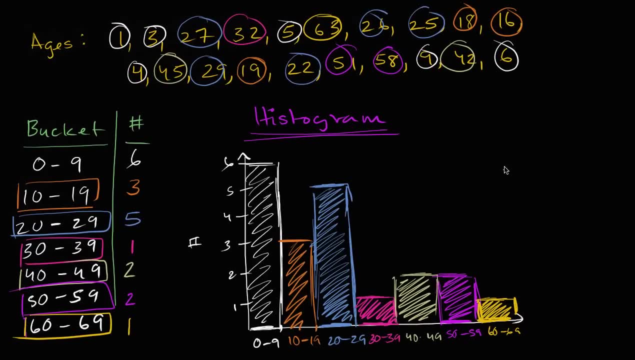 we have six people, And so you see that plotted out just like that, And obviously this doesn't apply just to ages of people in a restaurant. It applies to all sorts of data that you might want to collect and observe. 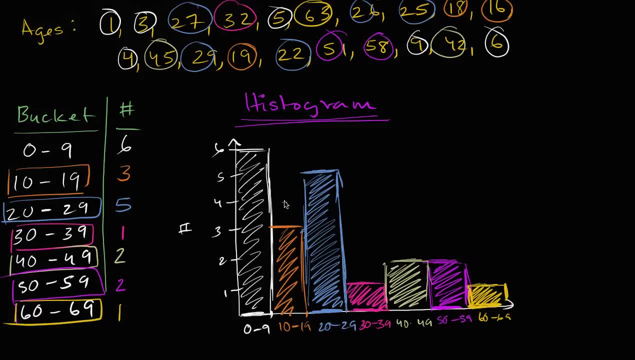 and they just bring a lot of kids to this restaurant. So it gives you a view of what's going on here. Just a lot of kids here, a lot fewer senior citizens. So once again, this is just a way of visualizing things. 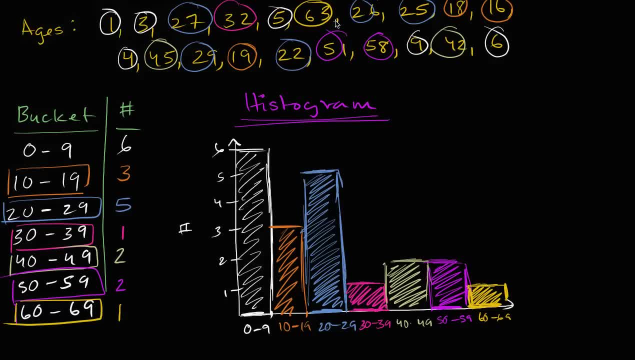 We took a lot of data. that can take multiple data points, Instead of plotting each data point like we might do in a dot plot. instead of saying how many one-year-olds are there, Well, there's only one one-year-old- How many three-year-olds are there?